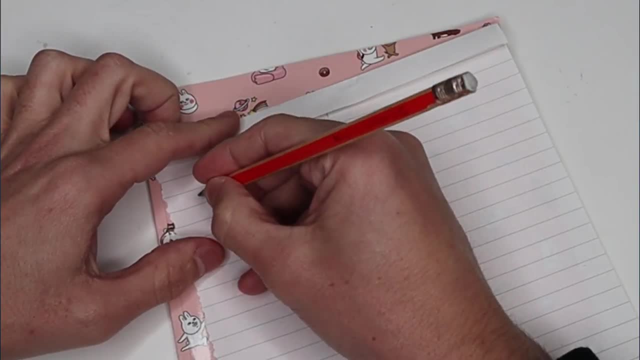 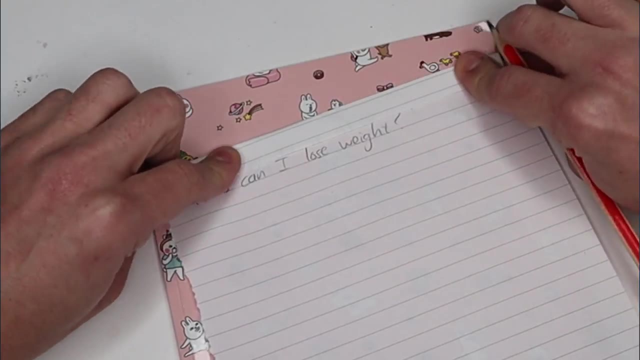 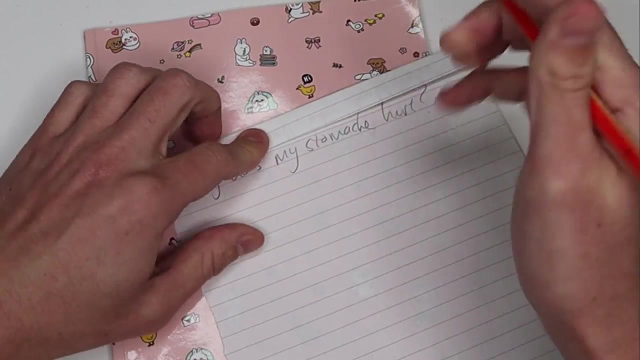 then pass it on to the person on their left. This step is tricky but interesting. Every writer has to write a possible question. after reading the previous answer they see in the paper. The same rounds continue till the bottom of the page and end with an answer. 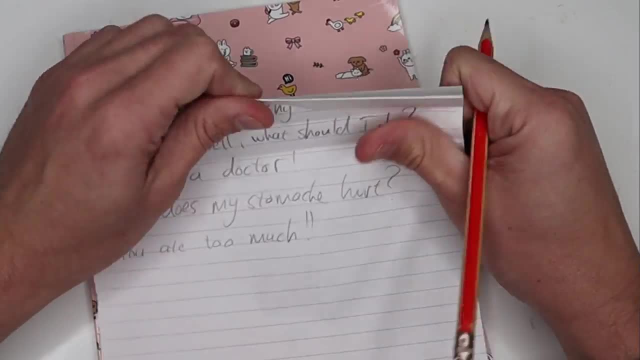 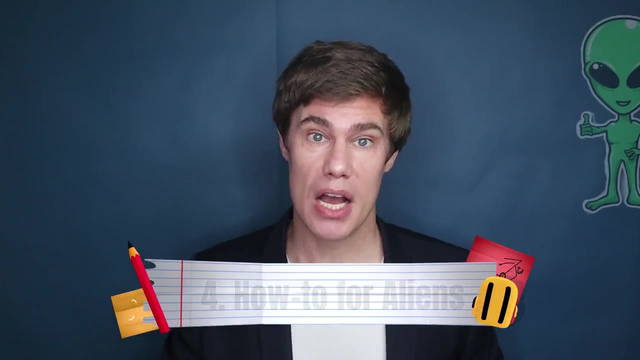 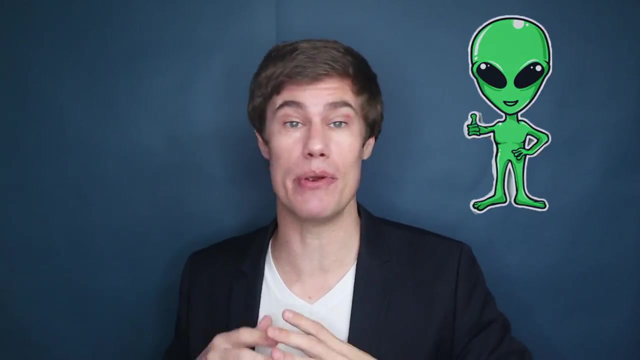 All the writers unfold their papers to read their original question, the answers they've received and everything in between. Number four: a how-to paragraph for aliens. Students have to write clear instructions for an alien to impersonate them, For example, write clear instructions for the alien on how to go to school. 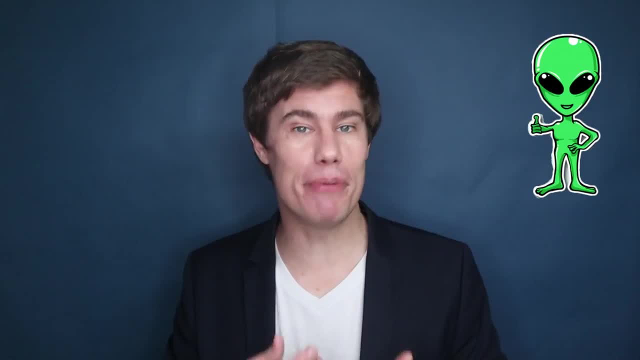 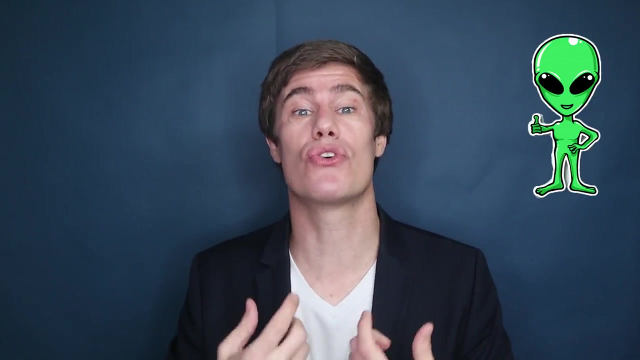 The alien should be able to impersonate you exactly without getting caught. This assignment asks students to think over something that is second nature to them. They must break down actions and describe them. Students must not only think about what they do, but how they do it. 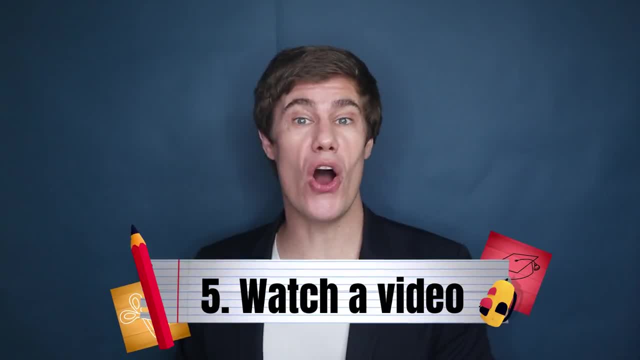 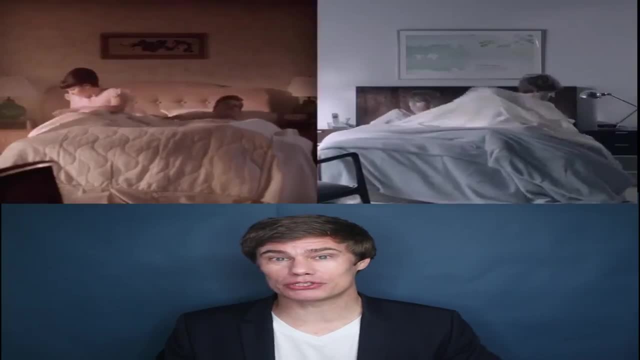 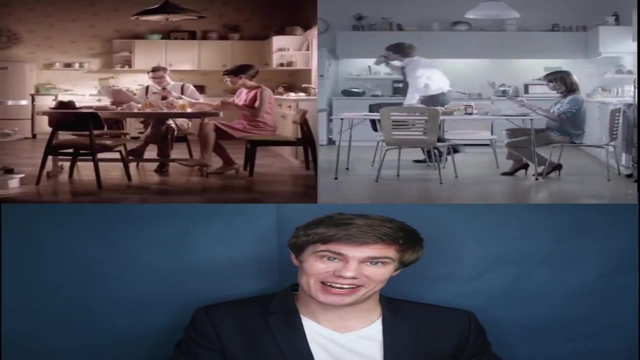 Number five: watch a video. You can use your own video, But as an example I'll use this one. It's from Coca-Cola and it displays the differences between today's life and the past by showing a grandfather and grandson's life side by side. 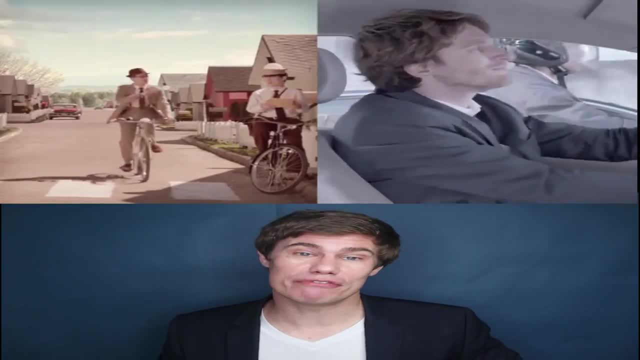 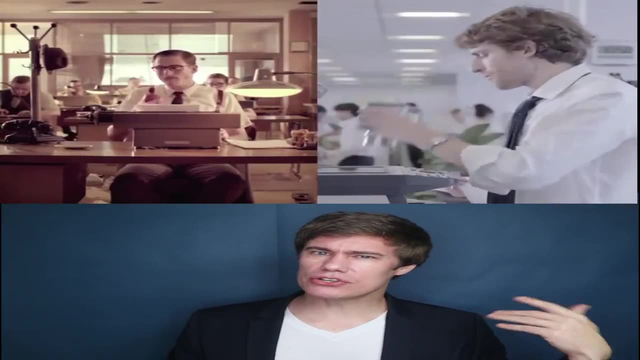 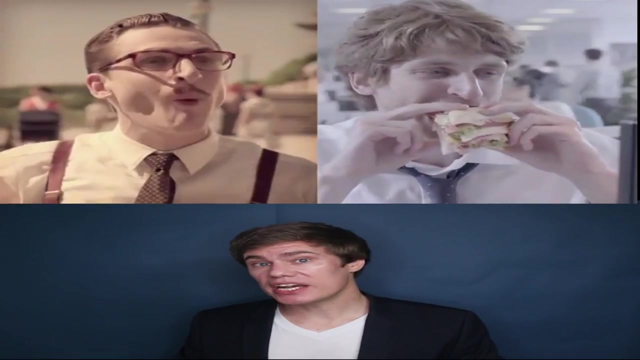 First put the students into pairs and then they watch the video. Then ask them questions. Start easy: What's your favorite drink? What did you see in the video? What differences were there? How is your life different from your grandparents? Then watch it again. 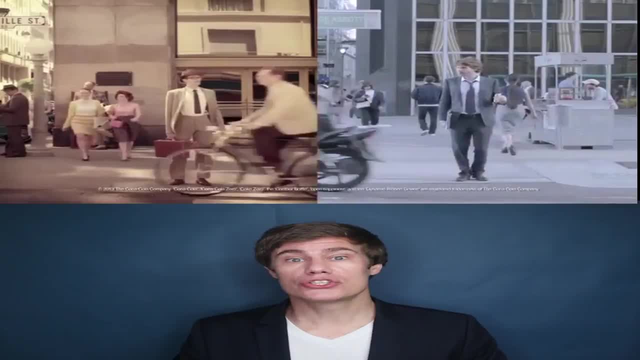 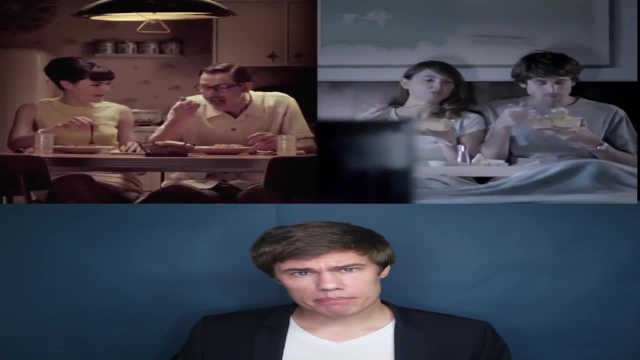 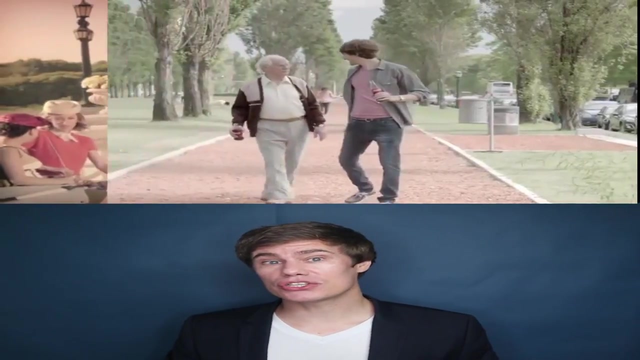 Each pair should write down the differences. they see Students construct sentences. Give them an example sentence. In the past people brought their lunch to work. Today people buy lunch. Finally, tell the students to apply some of the ideas from the board to write an essay. 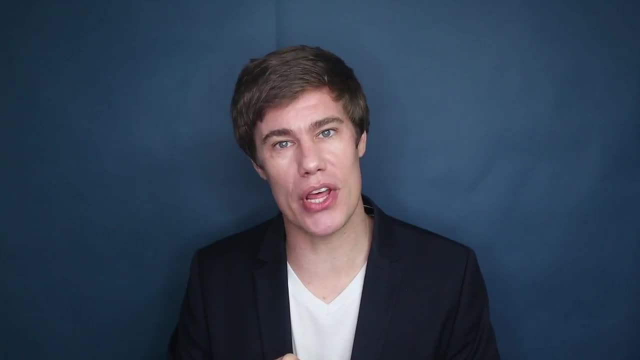 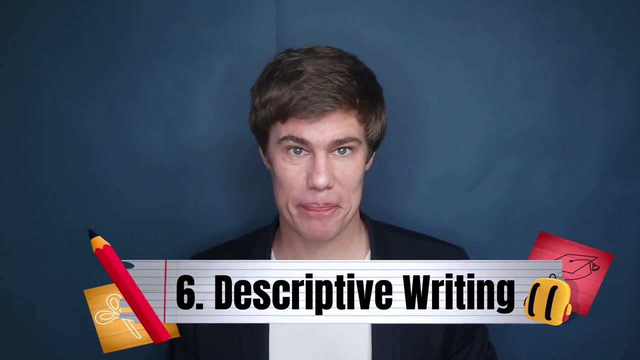 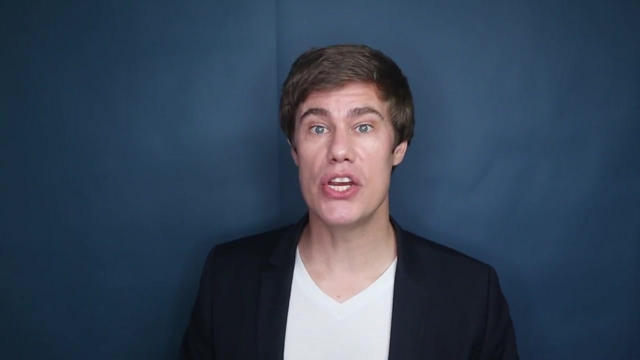 on how life has changed. Encourage them to use examples from their essay. Then ask them to write down the differences they see. Number six: Descriptive writing. The aim is for students to write about a single chosen object. In this exercise we use a cube to ask six kinds of questions about an item to help them. 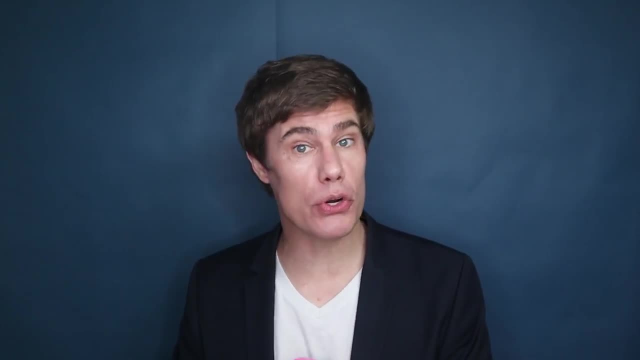 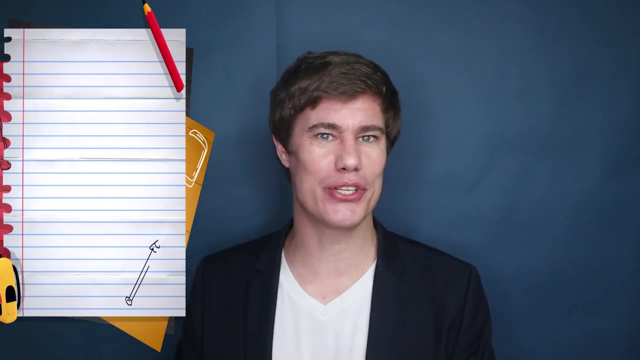 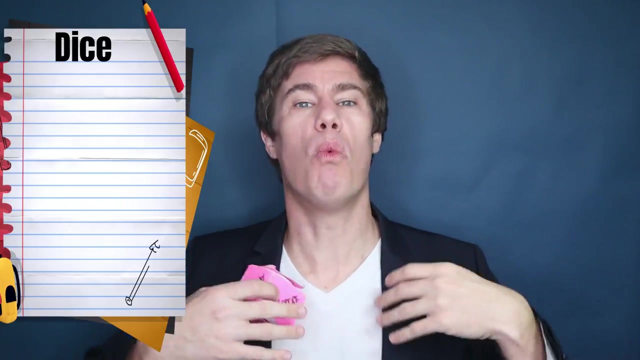 describe it. Each question gives students a different way to look at an idea or an object. The answers generate lots of information which helps students process the answer to their questions. detail to their writing: Describe What is the idea? What does the object look like? Describe: 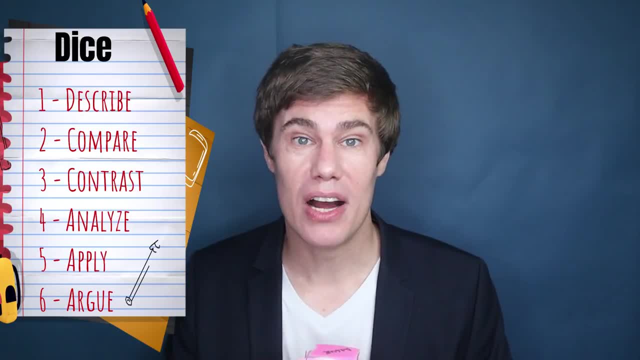 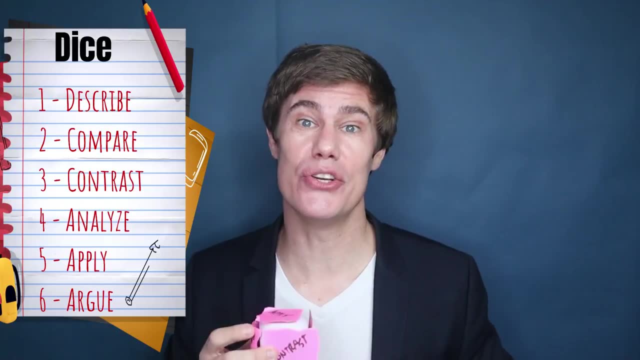 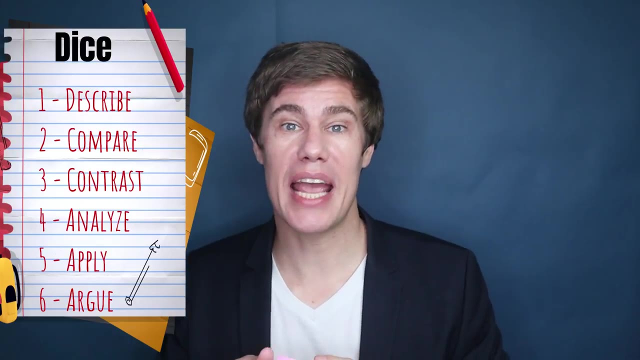 it with words about the senses. Compare: Is it similar to something else? Contrast: How is it different from others? What makes it unique? Analyze, Divide the whole thing into smaller parts, Apply. How can it be used, Who uses it, What can we learn from it? And argue, What do? 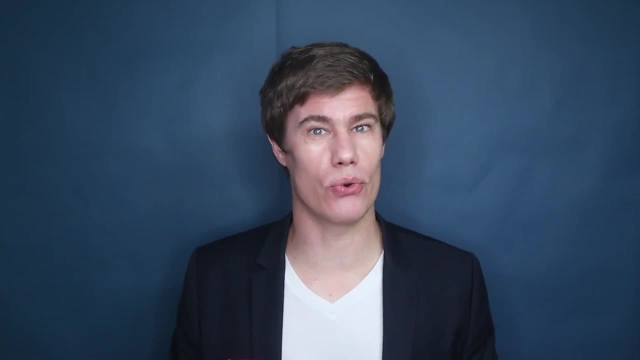 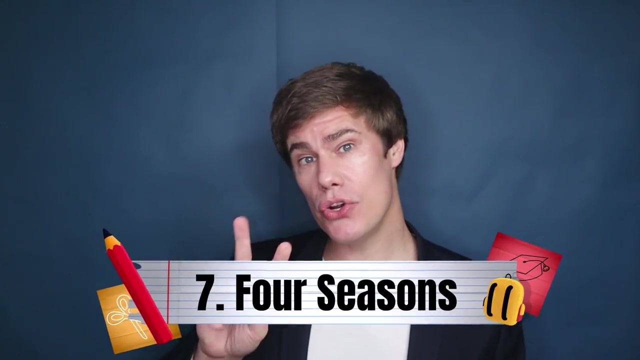 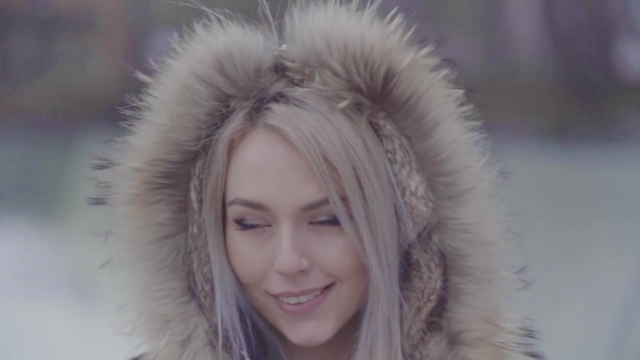 you think about it. Is it good, Is it bad, Right or wrong, Yes or no? Explain your decisions with reasons. Number seven: Four seasons In two link paragraphs. write about two seasons. Explain which season you like the most and which season you like the least. 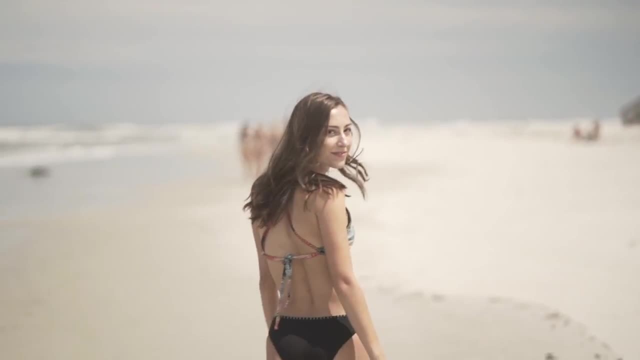 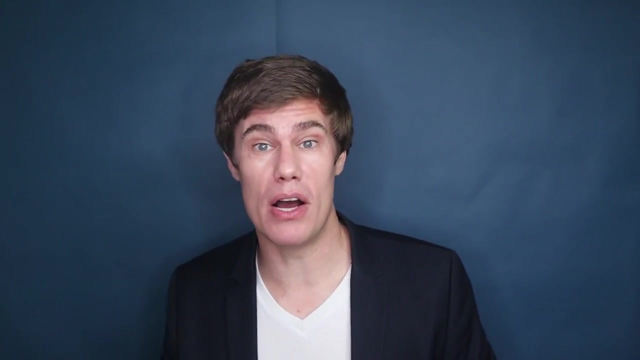 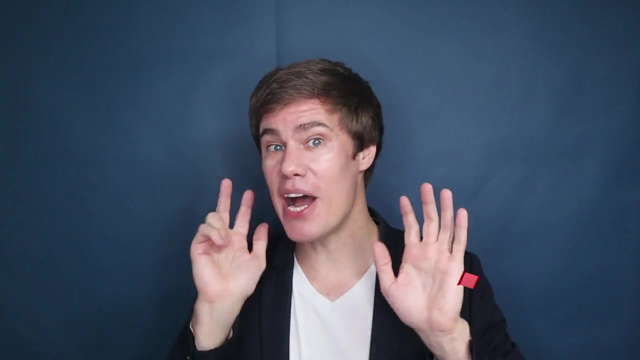 In order to help students write fully developed paragraphs, have them think of all the things they can write about. What do they do during summer but not winter? What is the weather like? Remind students to appeal to the reader's senses. Number eight Musical group writing Hand each. 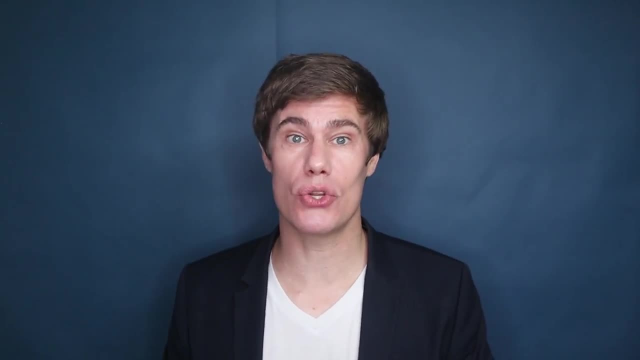 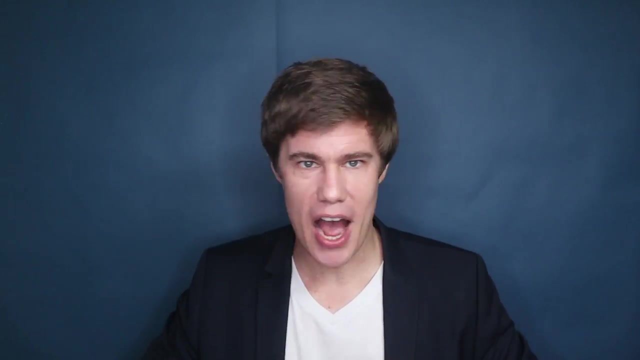 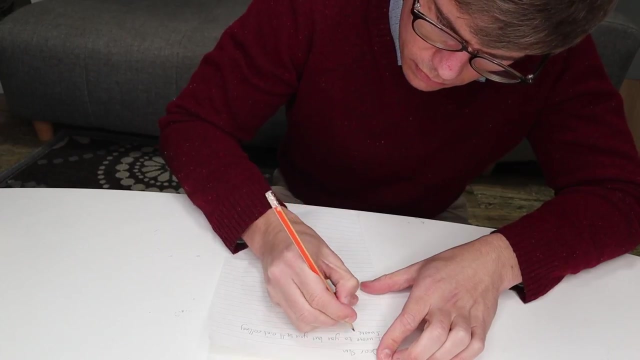 student a sheet of paper, Ask them to write a story from the top, Then play music and tell students to write accordingly. What is the mood of the music? African, drumming, Pop, Star Wars, theme, Classical- Whatever works for you, They write any story they want. When you stop the music, they pass the paper to the person. 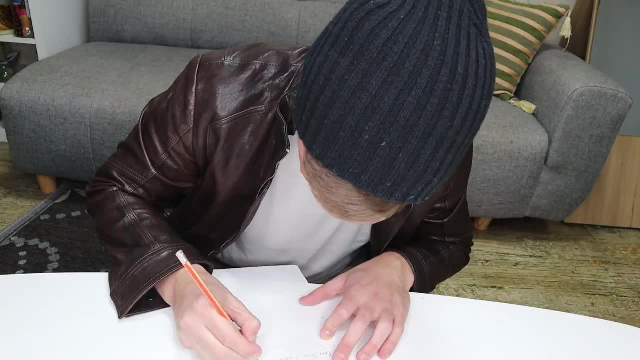 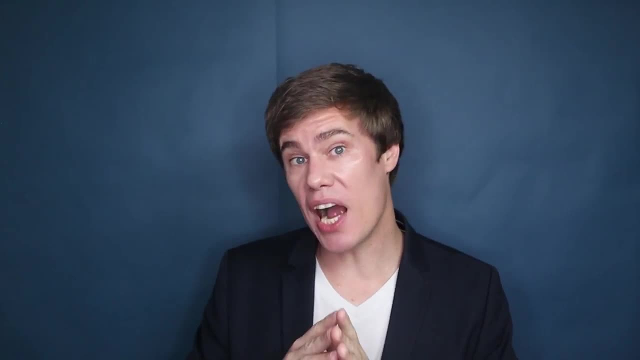 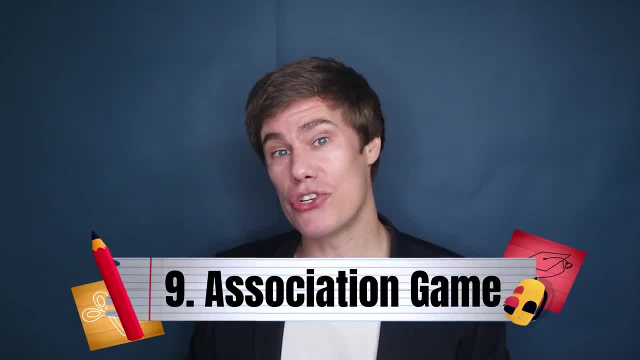 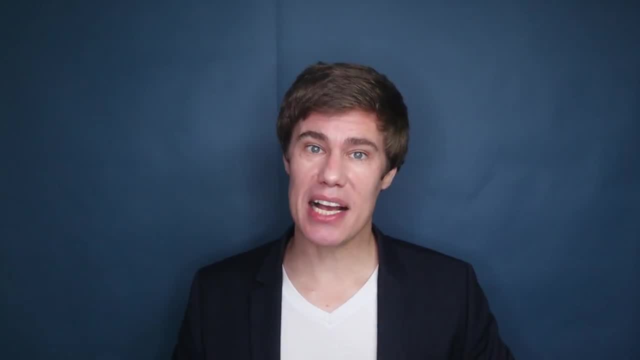 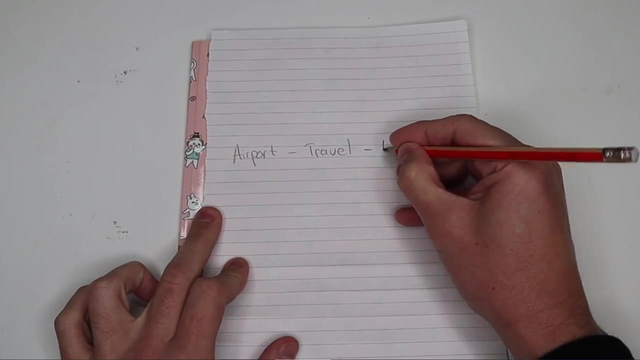